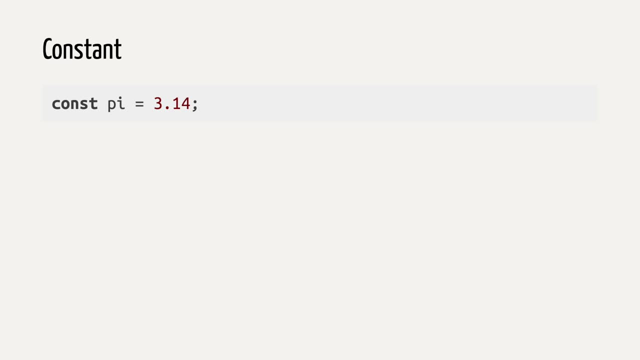 Last time we managed to simplify our calculation with constants. We have created a constant for pi and used it when finding out the surface area of different planets. This way we have reduced the amount of code, but we still have lots of repetitions. A line of code is called a statement. 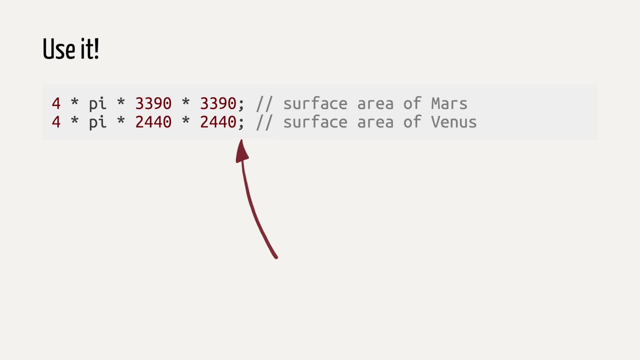 and statements in javascript should end with a semicolon. Here we have two statements and we still have to repeat the whole formula in each statement. And remember, we don't want to repeat stuff in our programs. It'd be cool if we had some sort of a separate special machine that. 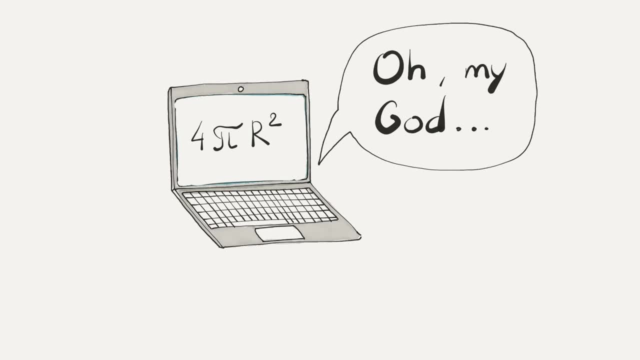 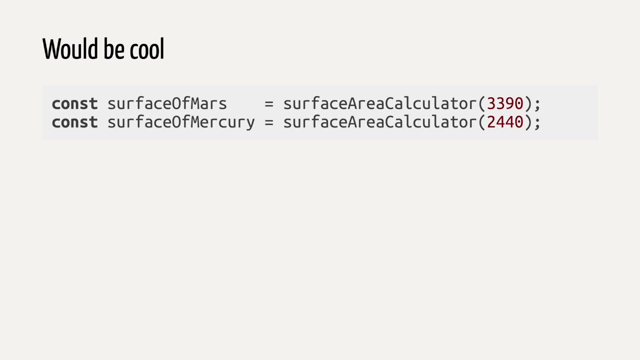 calculates the surface area of any given sphere. so that we could do something like this: Just tell it, hey, surface area calculator, give me the surface area of a sphere of radius 3390.. And it just gives you the answer. Well, good news, we can actually create machines like this. They are. 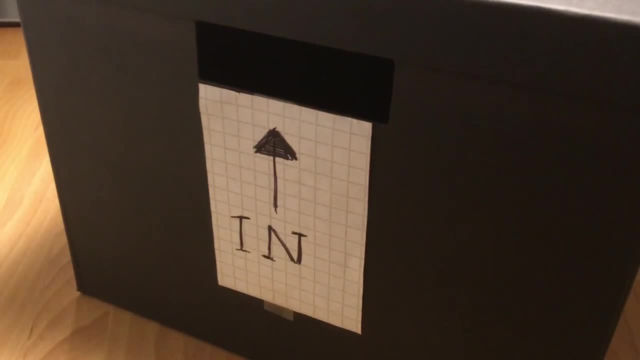 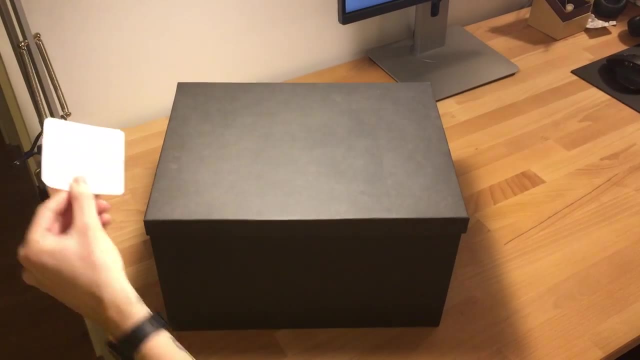 called functions and you can think of them as black boxes. Put something in inside the box and the box spits out something else. In this case, surface area calculator box would take in one number, the radius, and spit out another number, the surface area. 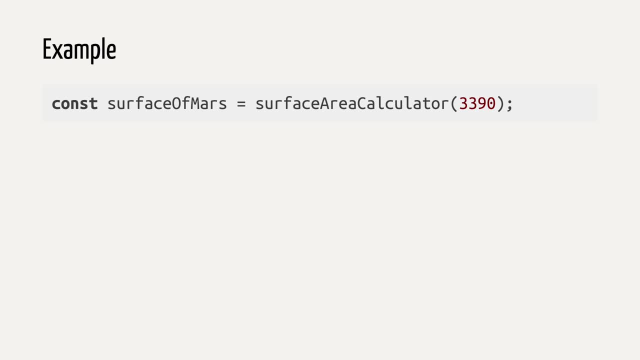 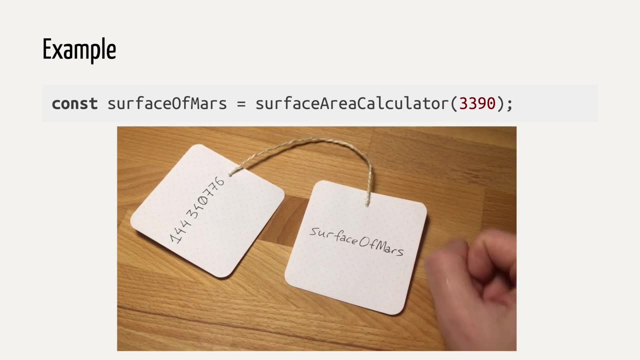 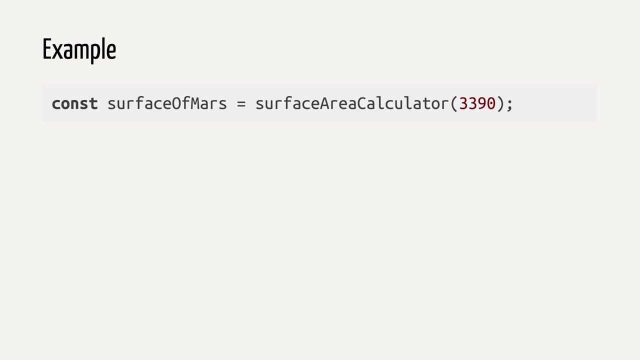 So in this example we are calling the surface area calculator box, giving it 3390 and getting back the answer. This answer is then stored in the surface of Mars constant. It's important to understand the difference between two things: Defining a function and calling a function. 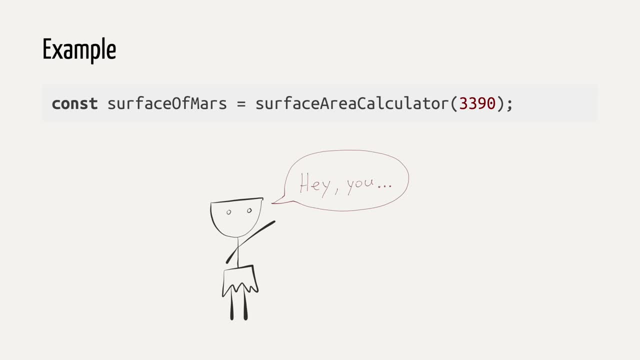 What we did just now was calling. We called the surface area calculator function. In other words, we assumed it already exists and we used it, But it has to exist, So we have to create it. before calling, We have to define the surface area calculator function. This 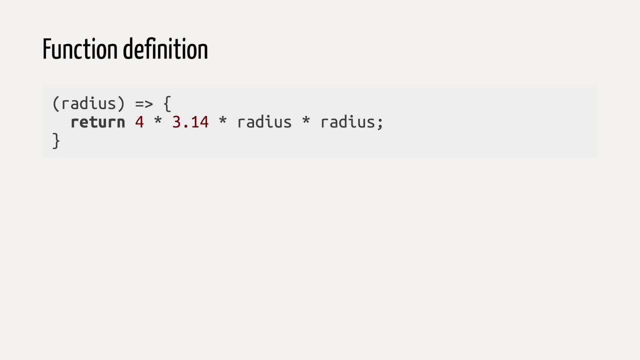 is the function definition. This structure with brackets- an arrow and curly brackets- denotes a function. This radius in brackets is how the function will refer to the number we pass in. In other words, radius is the name for the number that exists inside the function. when 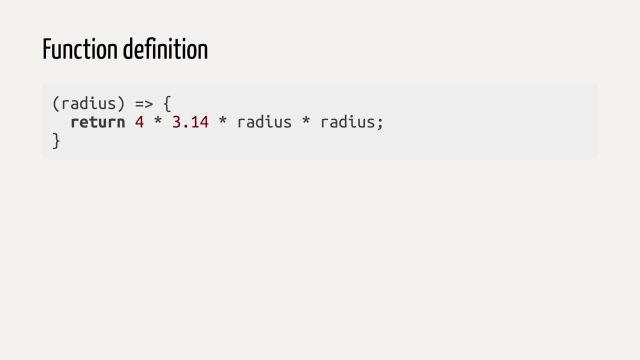 we call it. It's an argument of the function. This particular function takes in one argument, but other functions may take more arguments or take no arguments at all. The curly brackets create a block. You'll see blocks a lot in JavaScript and other languages too. They create. 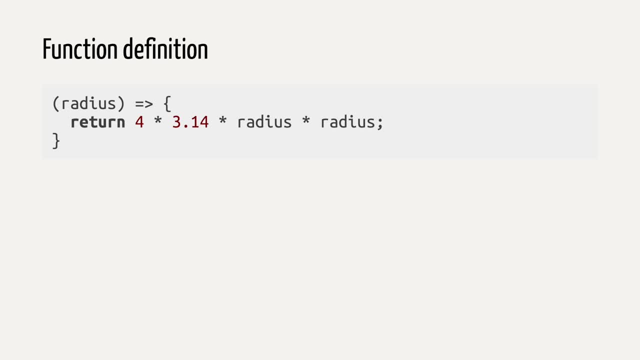 a group of statements And this is how we know where the function starts and ends. This function only has one statement. It starts with return And then you see the already familiar formula. You probably already guessed that return makes the box spit out the result, The result of the calculation 4 times pi, times radius. 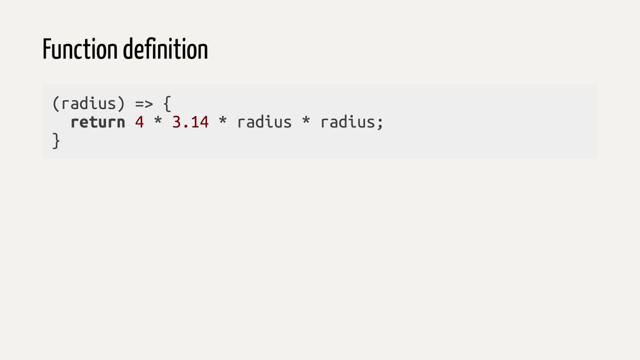 times radius is what the function returns to us after we call it. Now we need to give this function some name so that we can call it by name. I want it to be surface area calculator, but you can give any function, any name. There are certain rules, like the name cannot have. 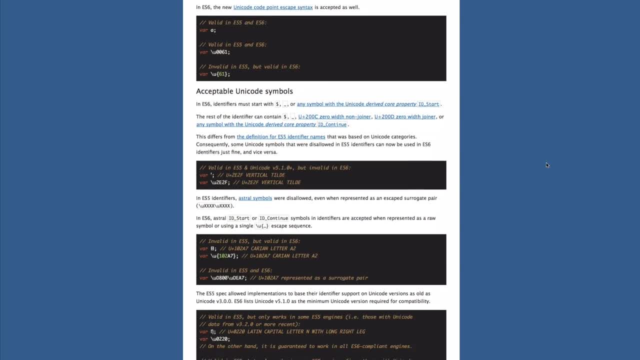 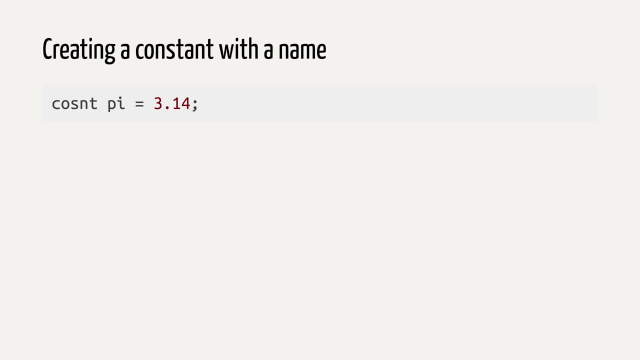 spaces in it and you cannot use some special words like const, for example, but otherwise you can call your functions and your constants as you like. We already know how to give numbers a name by creating a constant. It's exactly the same way with functions: Const, the name you want, the equal. 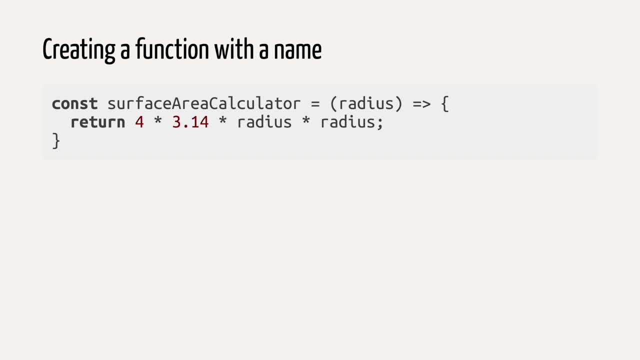 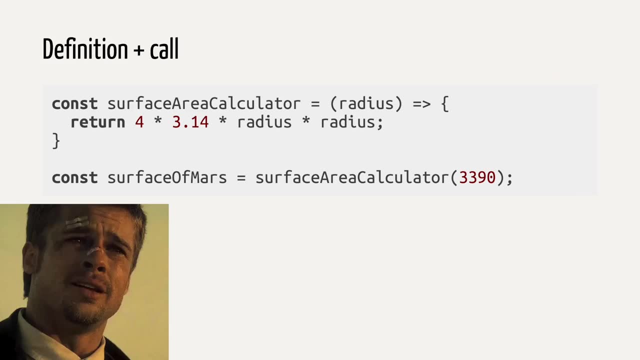 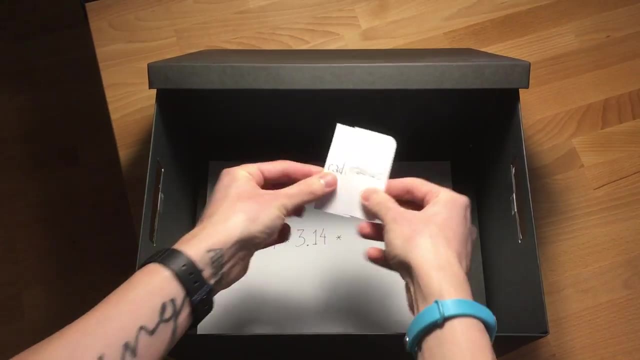 sign and then goes the function itself. So let's bring everything together. At the top there is a function definition and then we have a function call. Let's look inside the box. What's happening when it's called with 3390 as an argument. Return wants to return the result, but it's not ready yet. 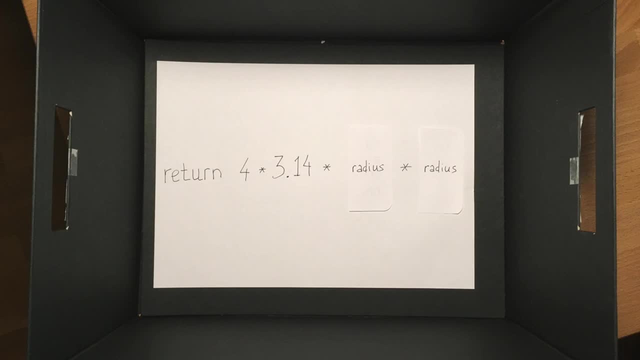 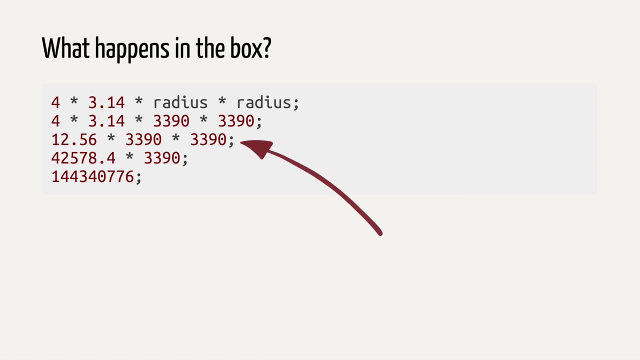 Calculations should happen first. The argument is used in the calculation, so first it needs to replace the name radius with the actual value that was passed in, and then do the multiplications, And 14430776 is then returned. You can also imagine what happens outside when our function. 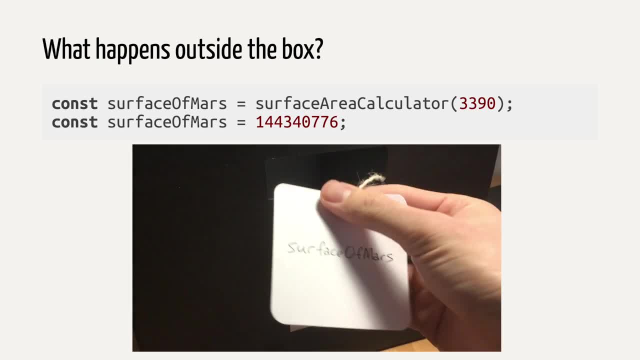 returns the value. Now, surface of Mars is a function that returns the value of the value of the function. So let's say that we have a function that returns the value of the function. Now, surface of Mars is a function that returns the value of the function. Now, surface of Mars is a. 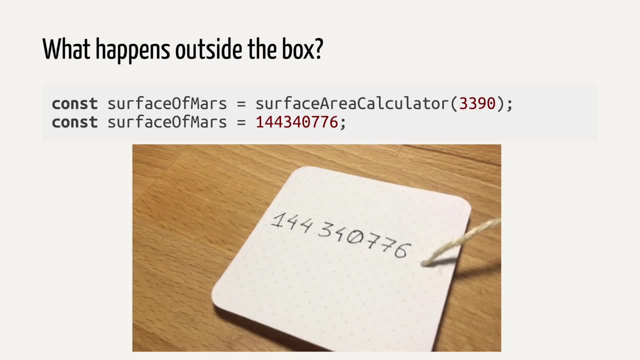 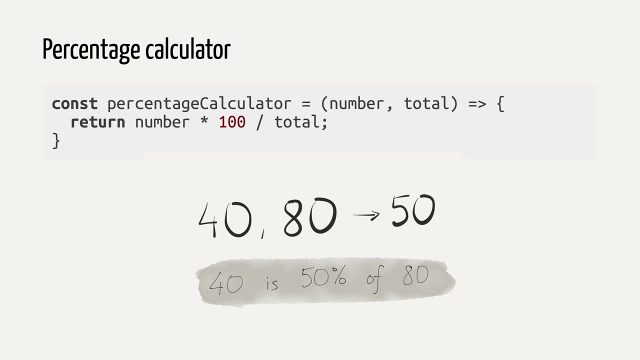 constant with a certain numeric value. Let's take a look at another example. This function takes two numbers and returns the percentage. If you give it 40 and 80, it will return 50, because 40 is 50% of 80.. As you see, when there are multiple arguments, they are separated by commas. 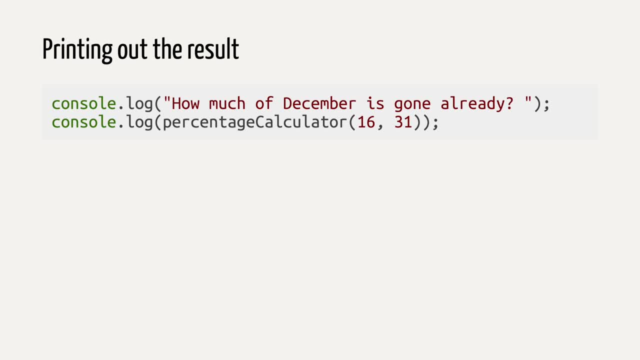 Let's print the result onto the screen. Today is December 16th and I want to know what percentage of December is already gone. Look at the second statement. There are two important points here. First, we can put the function call in any place where we can put a string.